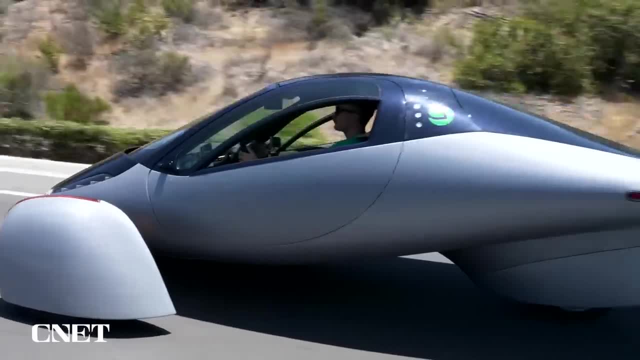 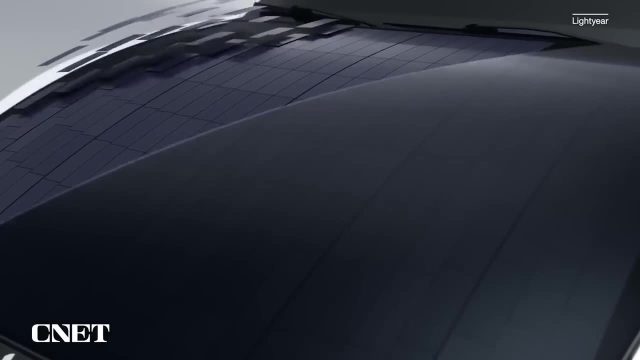 a solar EV last year when I checked out the Aptera. Most solar cars, like the Aptera, Sono, Scion and the Lightyear Zero, are engineered to be as light as possible so they can maximize the benefit from their solar panels. Also, it's important to note that solar cars don't 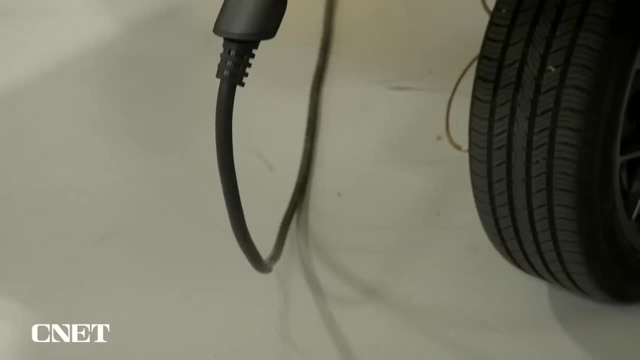 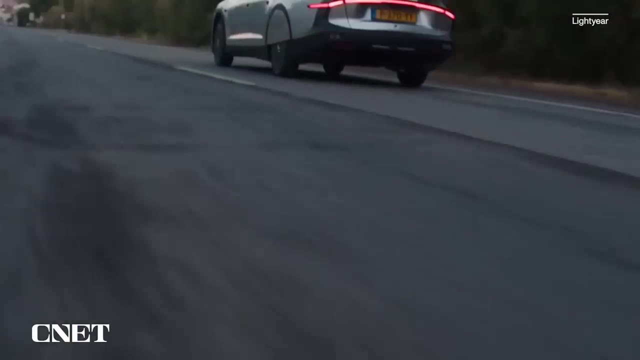 completely run on solar. They still need to be plugged into the grid to charge up for longer rides, But having solar panels all over your car could still provide up to about 40 miles a day, depending on the car, where you park it and what kind of solar package you have. 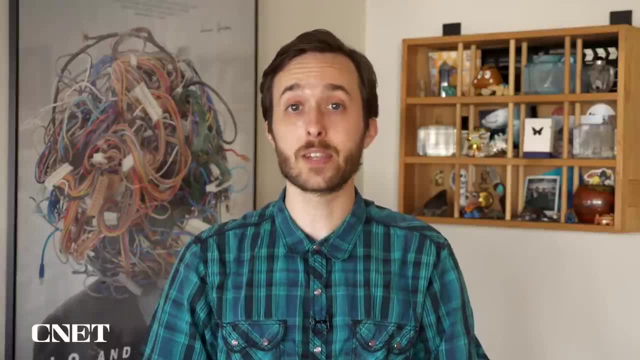 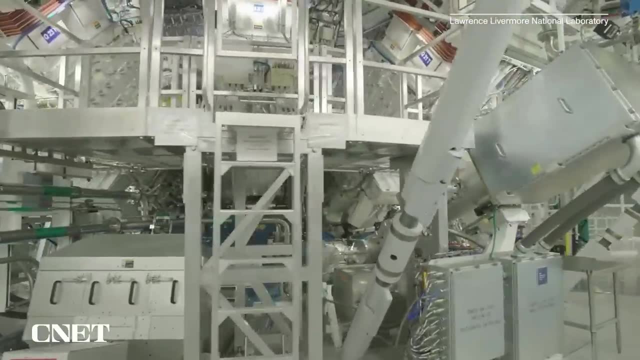 Capturing the sun's power is one thing, but there are actually people trying to replicate the sun's power here on Earth. I'm talking about fusion energy, which seeks to fuse elements together to generate energy, like the types of reactions occurring within the massive celestial. 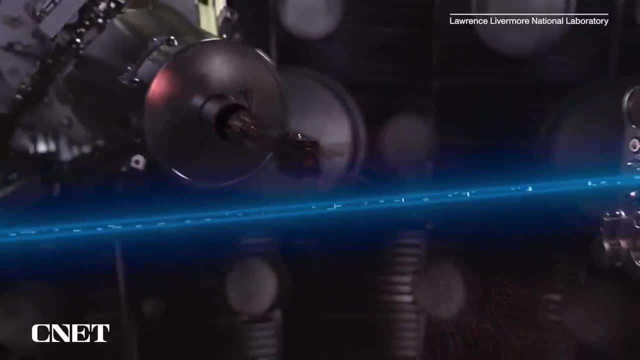 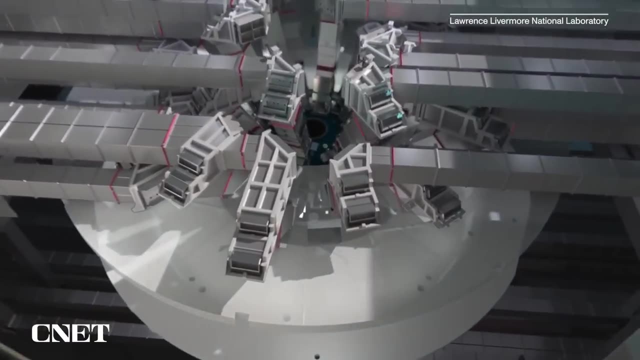 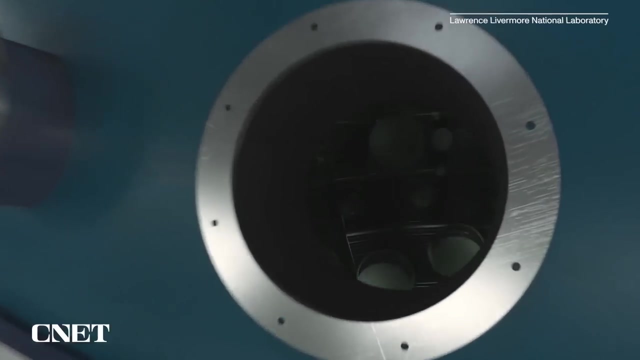 furnace we call the sun. Recently, a breakthrough occurred at the Lawrence Livermore National Laboratory, when a fusion reaction generated slightly more energy than what was required to start it, something which had never been done before. That said, fusion reactors still have a long way to go. It's likely they will need to be able to generate more energy than they. 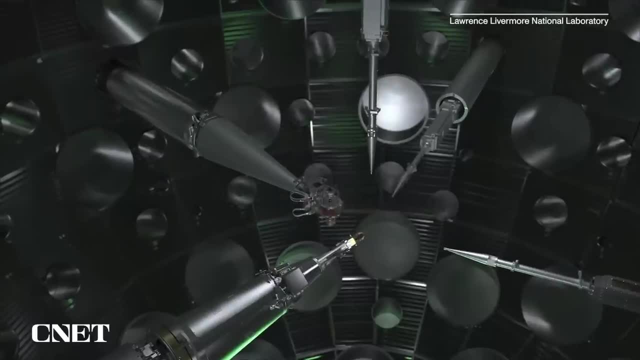 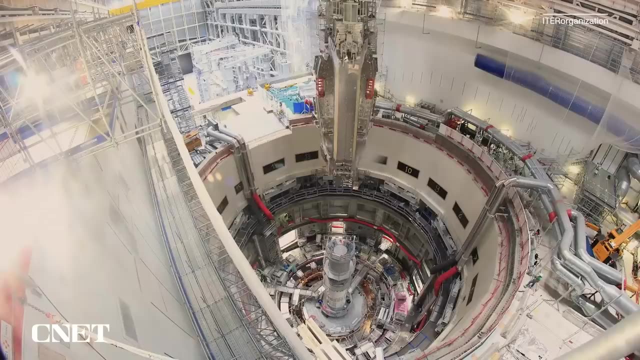 need to be able to generate 10 times the input energy to be a viable energy source, something which is still many years away, But with massive fusion projects like ITER on the horizon, there's a lot to watch in this space, and you can find it here on What the Future. 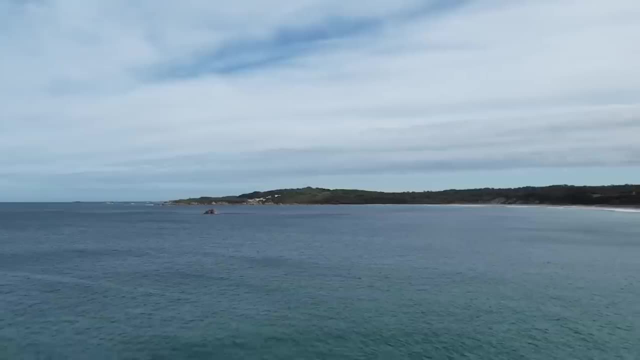 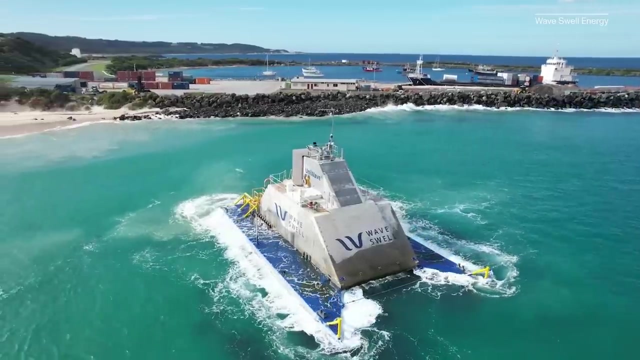 While solar and fusion take aim at harnessing the power of the sun, other energy tech companies are aiming at a power source a lot closer to home: the ocean. Waveswole Energy's artificial blowhole recently completed a one-year test off the coast of King. 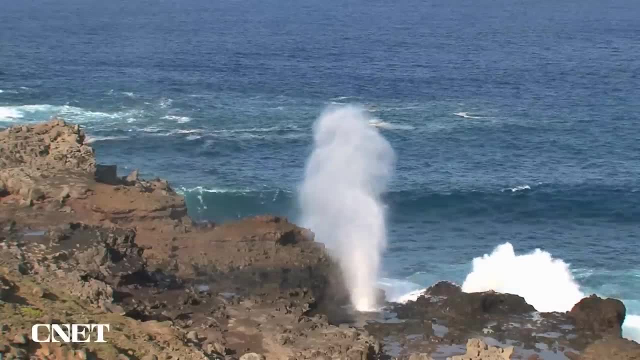 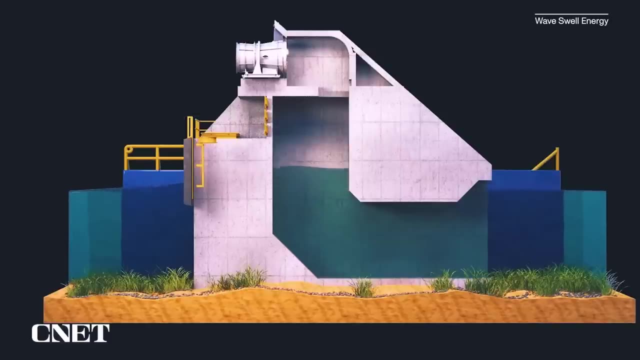 Island, Australia. Waveswole Energy's artificial blowhole recently completed a one-year test off the coast of King Island, Australia. Inspired by a natural blowhole, the Uniwave 200 directs waves into its central chamber, where air is compressed, spinning a turbine and sending energy to the grid. 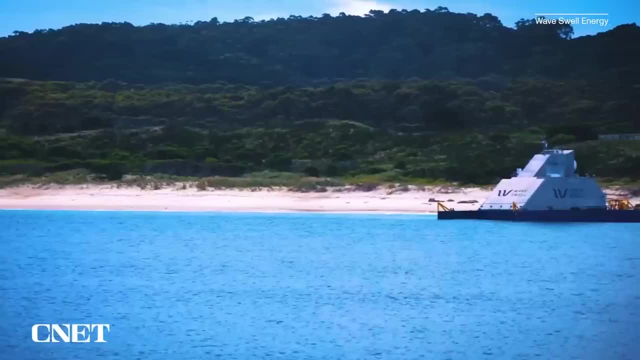 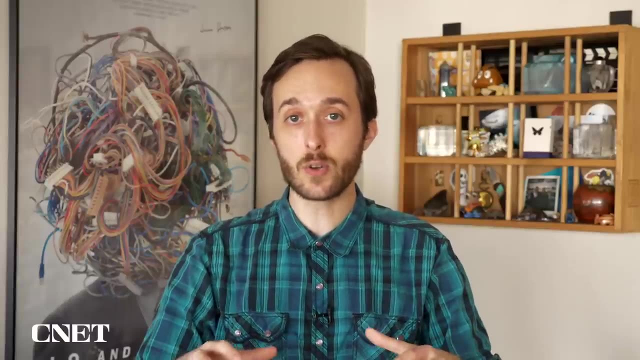 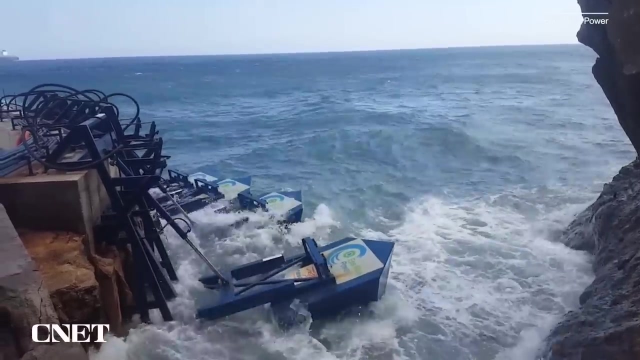 Waveswole Energy says it's still improving its artificial blowhole, making it more reliable and affordable. Another company called EcoWave Power is using man-made structures built into the ocean as a foundation for wave energy generation. These floaters sit on the surface where the rising waves push them up, creating fluid pressure.